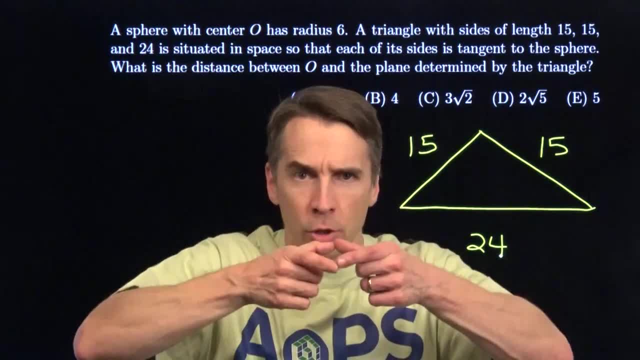 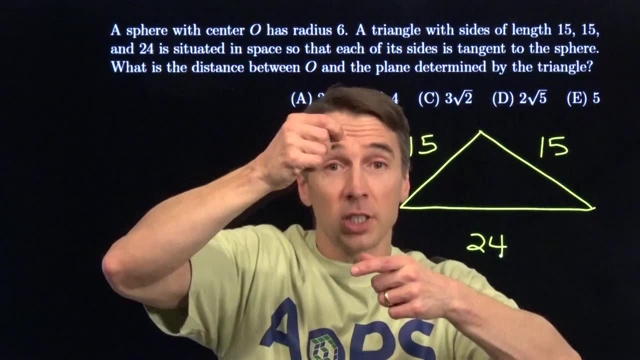 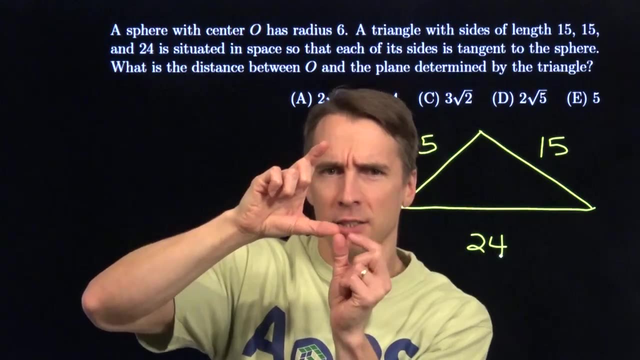 When you take the cross section of a sphere, you get a circle and the center of that circle, that's the point in the cross section that's closest to the center of the sphere. So there's the distance we want to find and the radius of that circle. put those two together, those 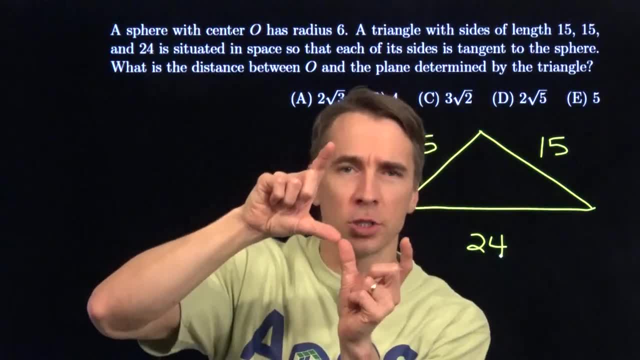 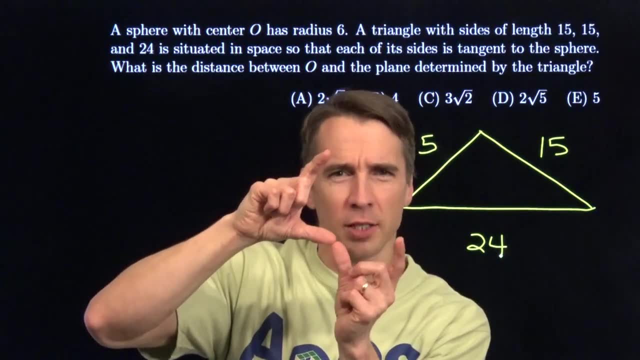 are legs of a right triangle and the hypotenuse is the radius of the sphere, and they told us that's 6.. So if we find the radius of this circle in the cross section, we can use the Pythagorean Theorem to solve the problem. 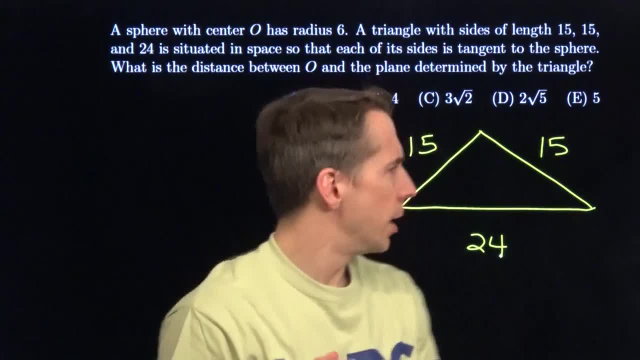 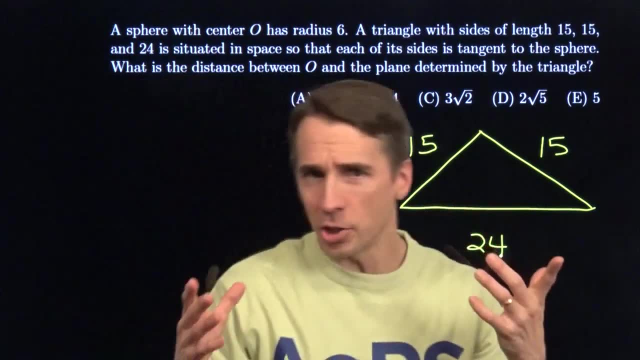 Alright, here we go. We've got to go after the radius of this circle, but where do we put the circle in this diagram? How's the triangle related to the circle? Now, in a triangle, all three sides are tangent to the sphere, so all three sides of the triangle. 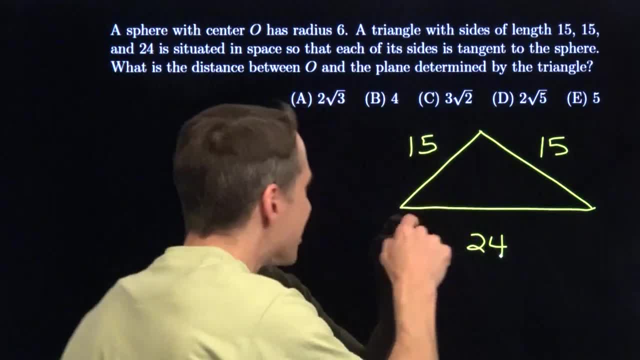 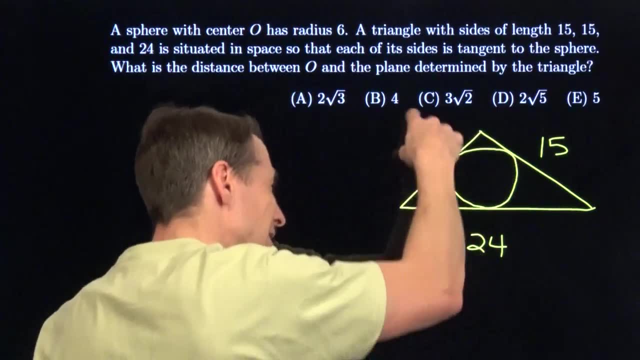 are tangent to the circle in the cross section. This circle is inscribed in this triangle. There it is, There it is. Now I see a circle, I see some tangents here. I'm drawing radii to those points of tangency. 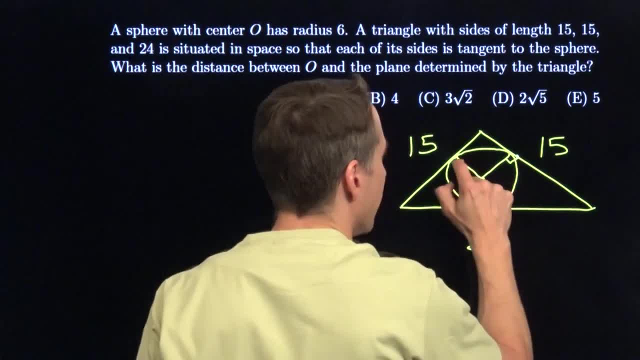 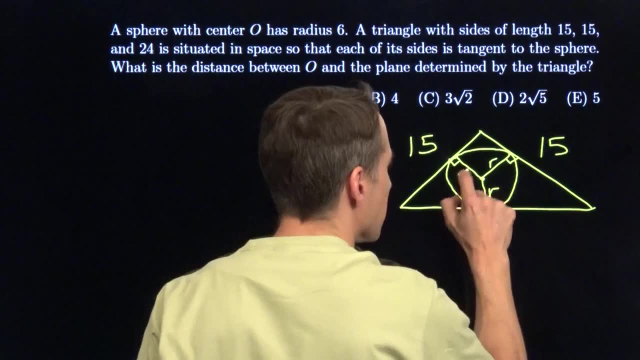 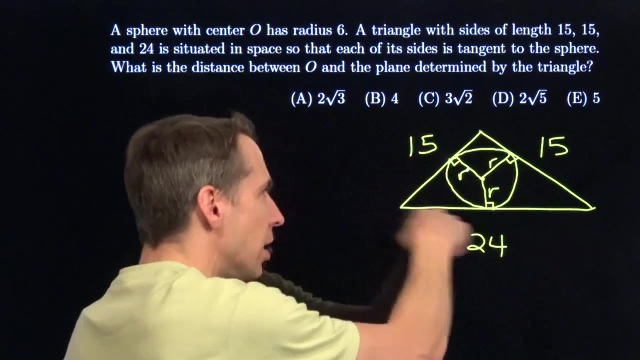 because that gives me right angles. I like right angles. Now I'm going to label each one of these r. we're going to use r for the radius of this circle, here and now. we're going to find r by using area, because you can find the area. 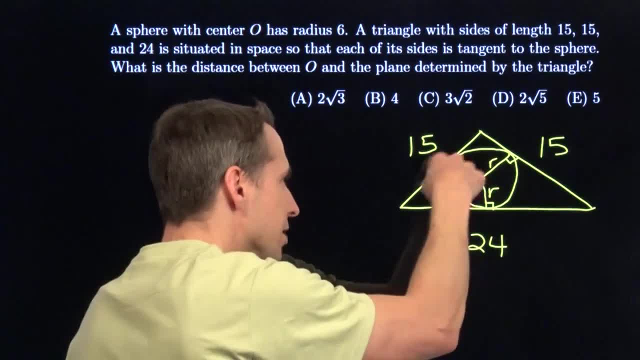 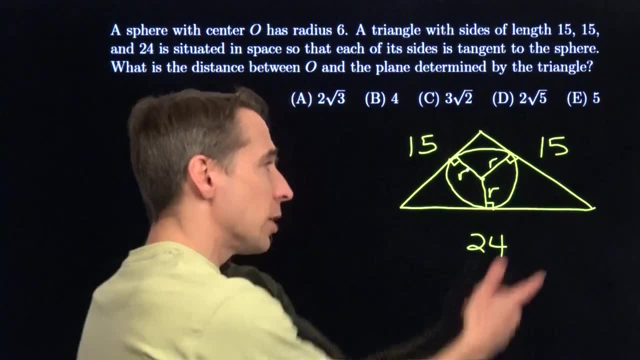 of a triangle by multiplying the radius of the circle that's inscribed in the triangle. It's inscribed in the triangle by half the perimeter and that'll give you the area. That's great, because we can also find the area of this triangle, because this triangle's 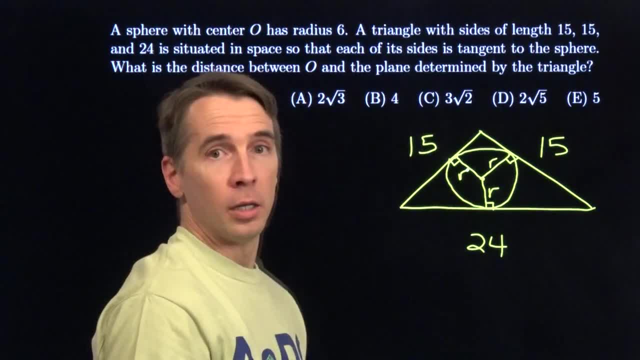 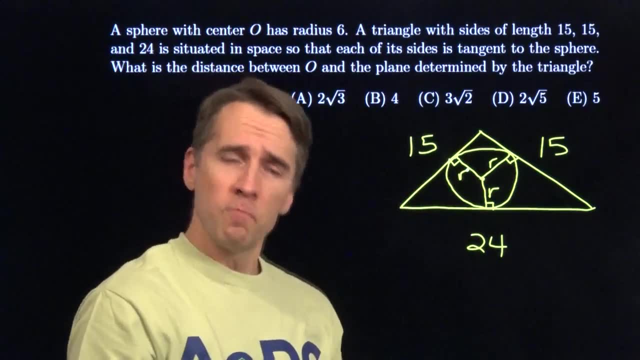 isosceles. We're going to drop an altitude to find the area. What's that? Oh, you don't buy that thing. I told you about using the radius of the circle to find the area of the triangle. That's cool, Let's prove it. Let's prove it: We're going to break this triangle. 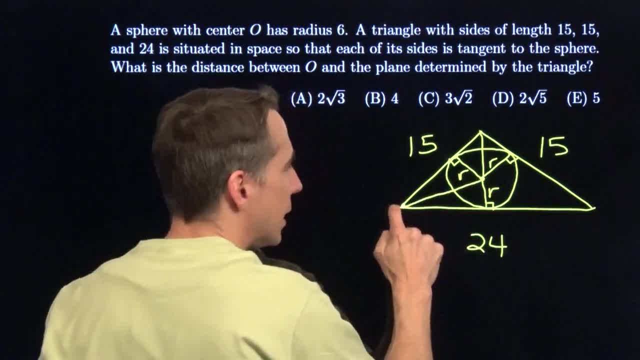 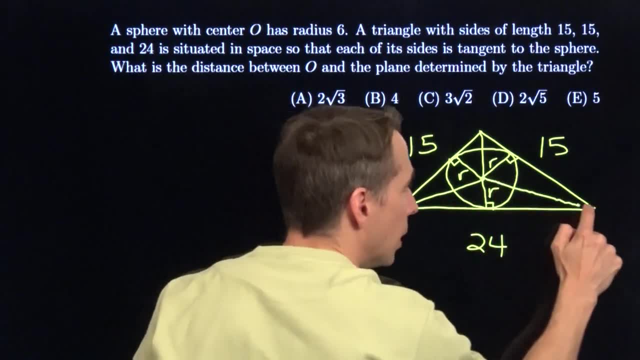 up into three smaller triangles. One's right here, over here on the left. It's along the side. Right there it's got altitude of the radius of that circle. Then we've got another one over here on the right, Same thing, One side's along the side of the original triangle, and 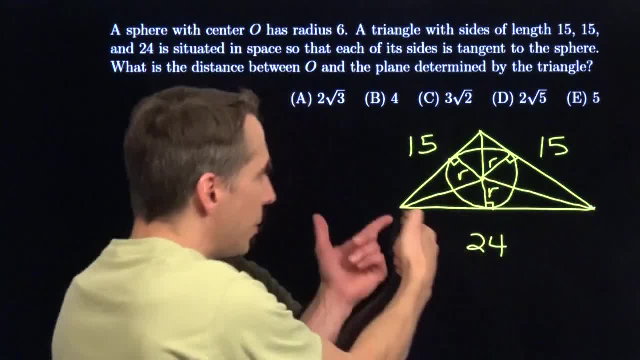 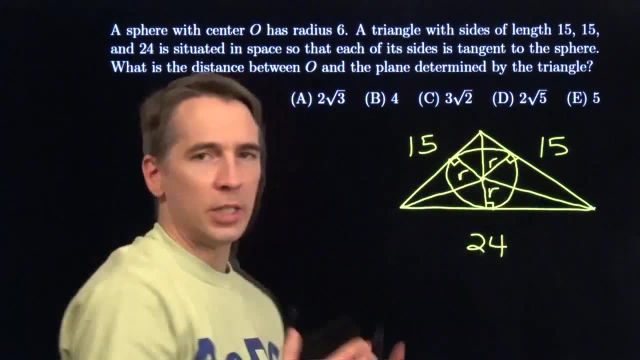 the altitude radius of the circle. Then down here on the bottom there's the third side of the triangle, altitude radius of the circle. So now we're going to add up the areas of these three triangles. That gives you the area of the whole triangle. Let's find those. 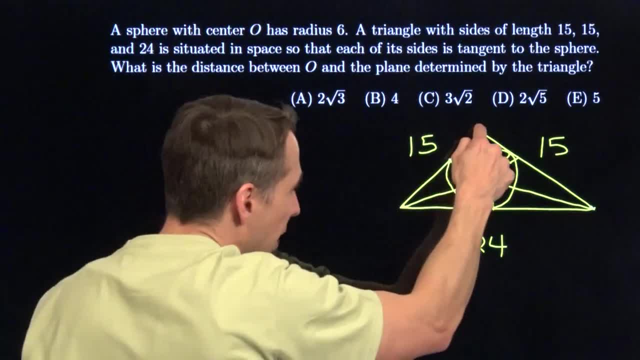 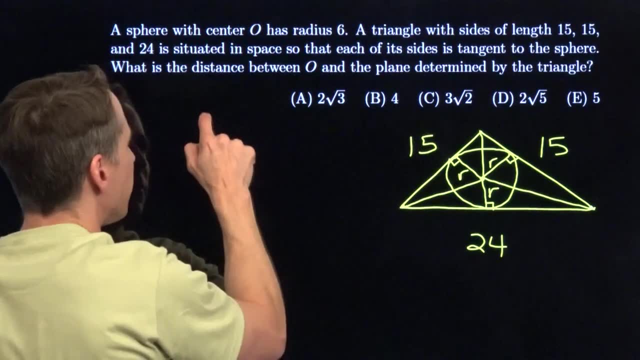 areas. in terms of the radius of the circle, In each case we have side of the triangle times radius of the circle, because that's the altitude right there divided by two. So we got a fifteen times r over two for this triangle right here. Same thing for the triangle. 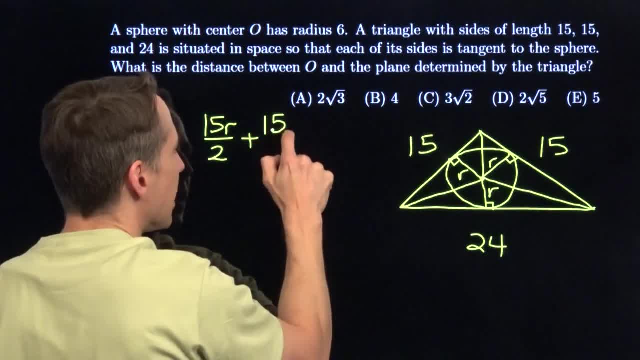 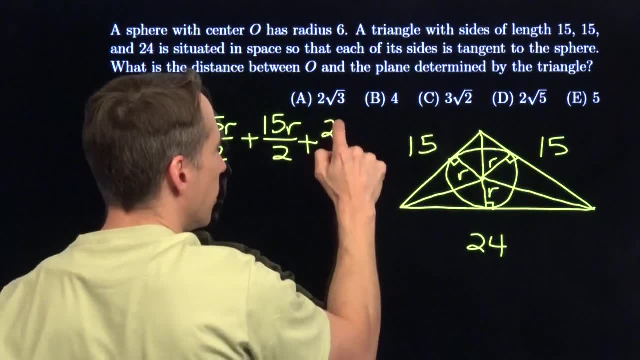 over there on the right, That gives us another fifteen times r over two. Then down here on the bottom we've got twenty-four times r over two. I know you're sitting there saying: but that's twelve r. Yes, it is, but I'm going to leave it like that for just a second, because 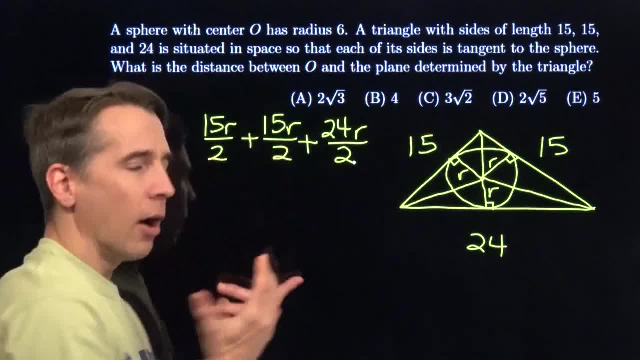 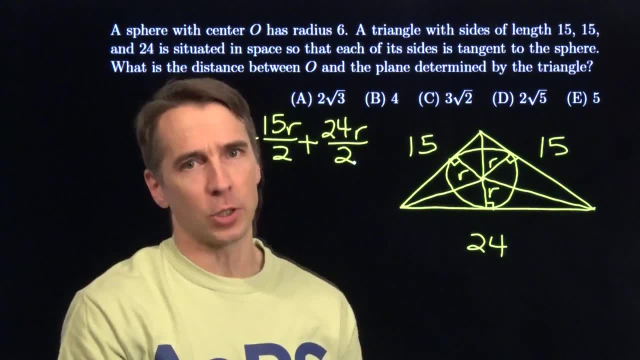 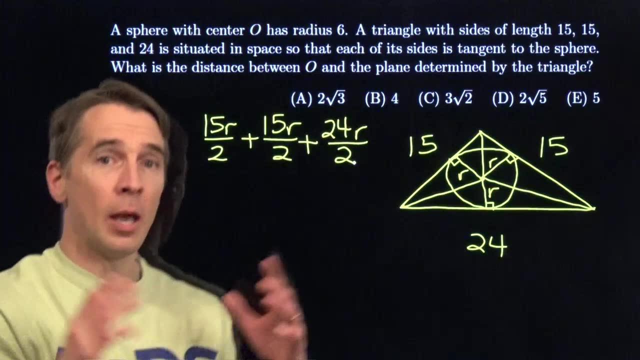 look what happens. We add up those numerators. We get r times the sum fifteen plus fifteen plus twenty-four. That sum is the perimeter of the triangle fifteen plus fifteen plus twenty-four. So this expression right here is what you get when you're going to be multiplying the radius. 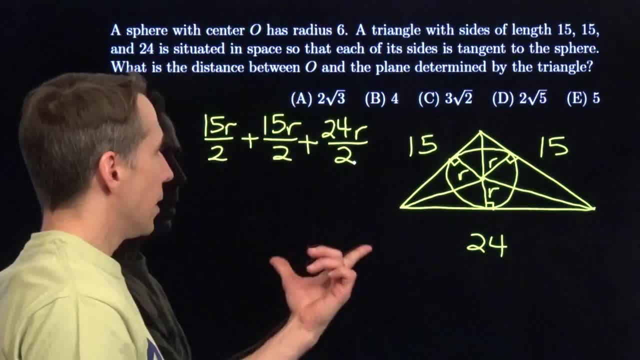 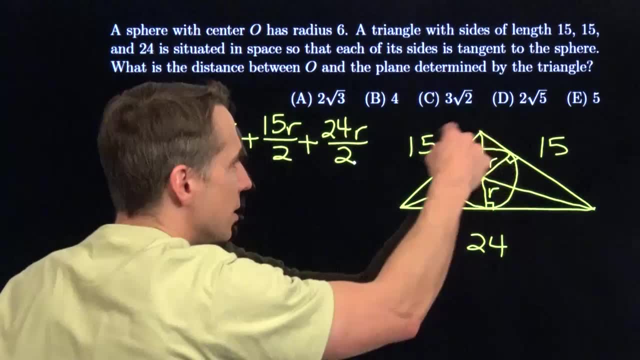 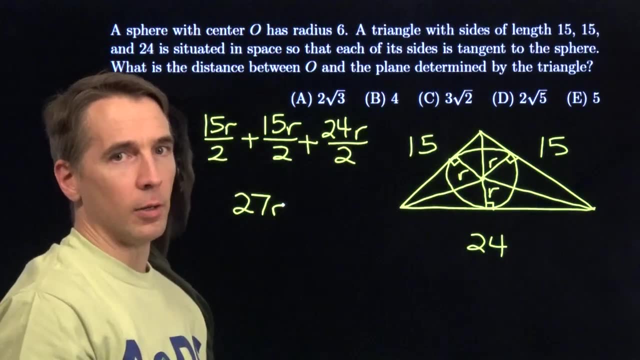 by the perimeter divided by two. Alright, let's do that. We've got the perimeter. fifteen plus fifteen plus twenty-four, That gives us fifty-four times the radius of this circle divided by two. That gives us twenty-six, That gives us twenty-seven r, And that is the area of this triangle And we can find. 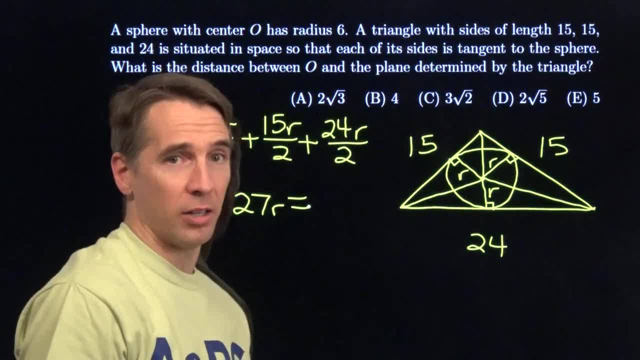 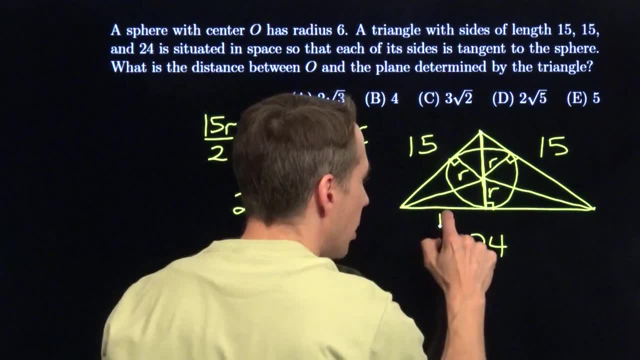 the area of this triangle. We can find the actual number. that's the area of this triangle. Just look at this altitude right here. It's an isosceles triangle. This altitude's going to split this base in half. Put a twelve over here, Put a twelve over there And this right. 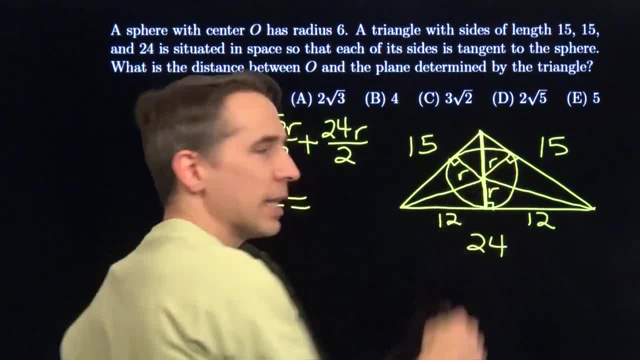 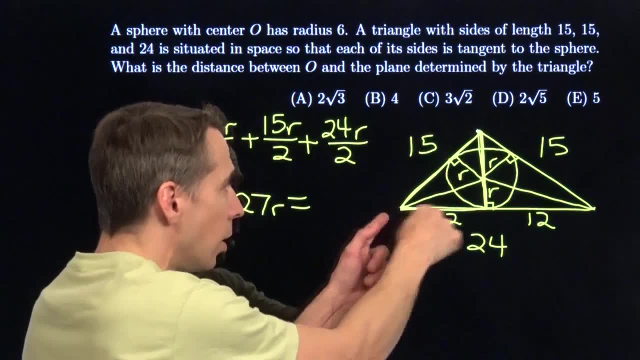 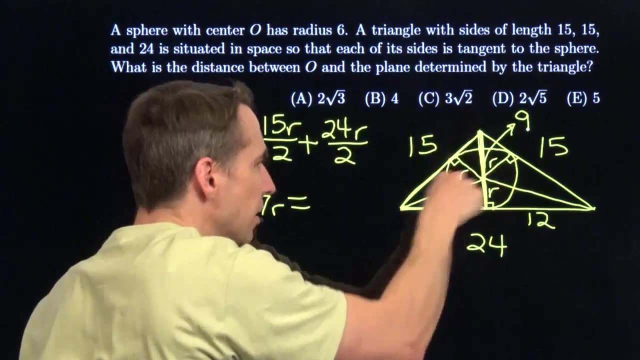 here is an altitude, And we can find what that is by breaking out the Pythagorean theorem on this triangle right there. Or we can just recognize: Hypotenuse is fifteen, One-eighth is twelve, One-leg is twelve, This leg right here is nine, And now we can use this nine. 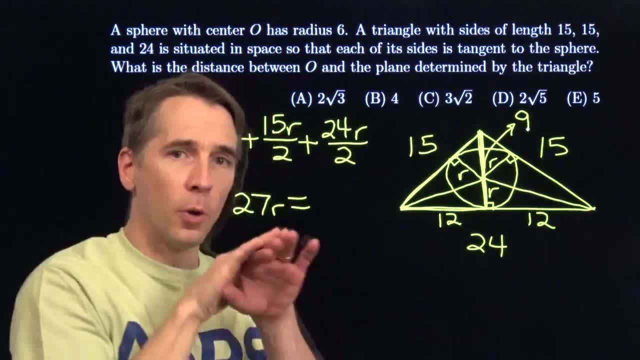 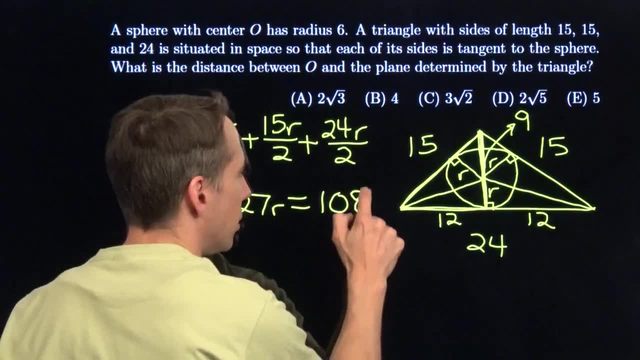 to find the area of the triangle. Nine times twenty-four divided by two. Twenty-four divided by two. We already did that. That's twelve. Nine times twelve is a hundred and eight. So the radius of this circle here we're just dividing by twenty-seven on both sides That.